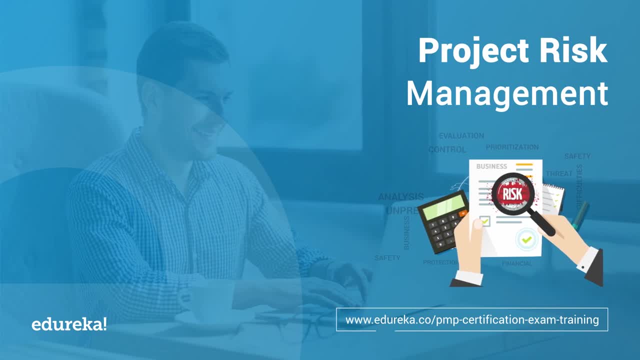 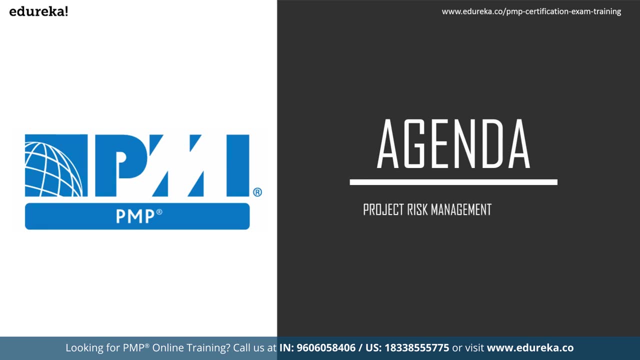 PMP, PRINCE2, Agile, Scrum, Master, DevOps and COVID-5.. The agenda of this webinar would be project risk management: understanding what is project risk management knowledge area is all about overview on risk management and risk management processes. So now, before we get, 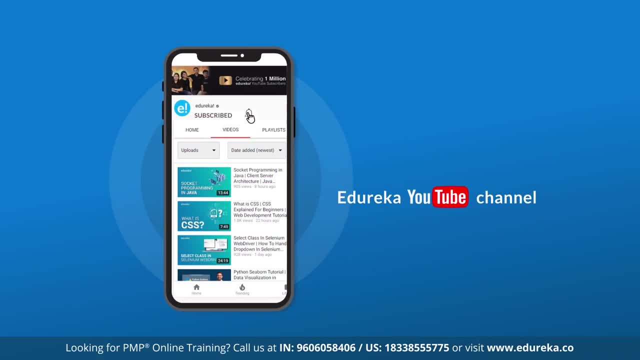 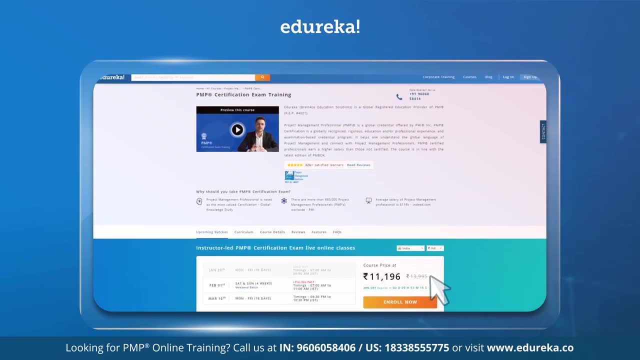 started. subscribe to Edureka YouTube channel and hit the bell icon to never miss an update from us on trending technologies. Also, if you're looking for an online training certification in PMP, check out the link in the description box below. Now, coming back to risk management, 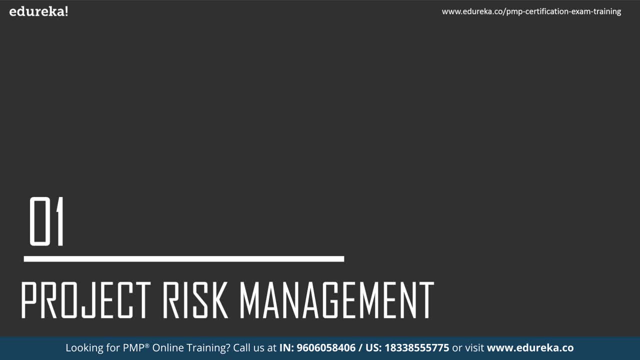 before we get into risk management, we should understand what is risk. So every project, every business, every investment done by an organization will be having certain kind of risks. So those risks needs to be managed. So what is risk? Risk refers to an uncertainty, Uncertainty. 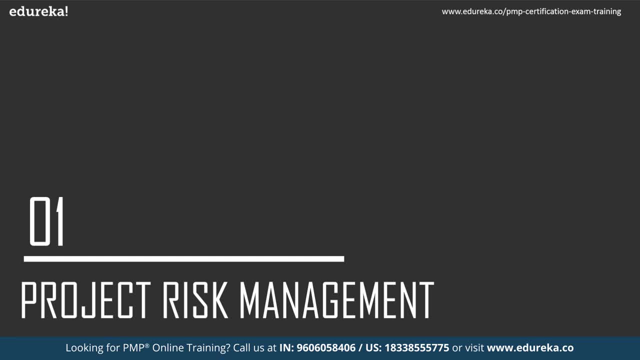 of an something, maybe positive or negative- which resides in the future. If that occurs, which becomes an issue to be handled, then it becomes an issue to be handled. If that occurs, then it becomes an issue to resolve. So the moment it occurs there will be some impacts. 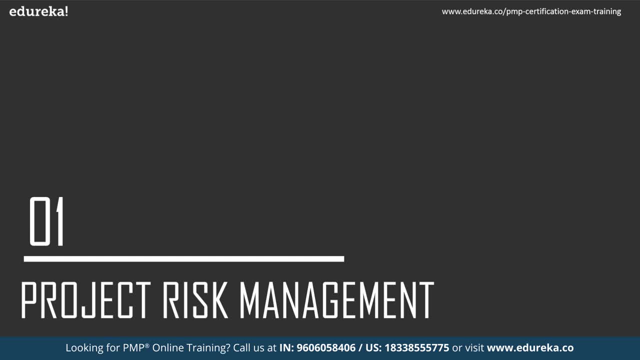 If it is negative impact, we call it as a threat. If it is positive, we call it as an opportunity. So, negative risk, which has a negative impact, which needs to be the impact of those, needs to be reduced or that needs to be eliminated or reduce the probability of that occurrence, by 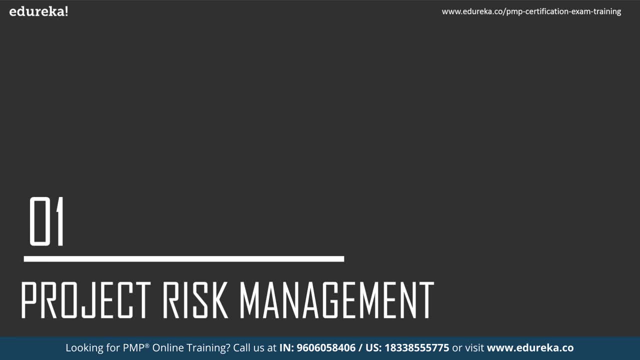 taking necessary actions or become ready. Yes, there is a risk. I cannot do anything about it. To reduce the impact of that risk, I will become ready to do something when it occurs. If it is positive risk, I will take the advantages of that. I exploit that risk, I enhance. 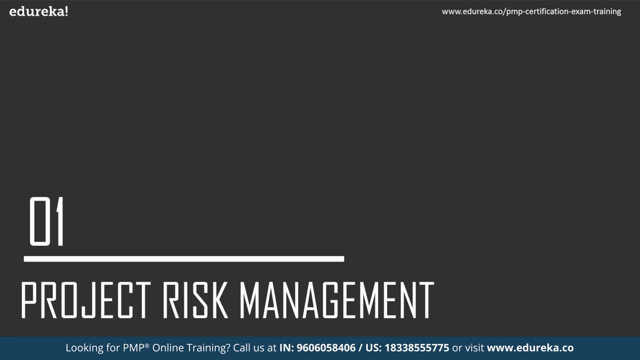 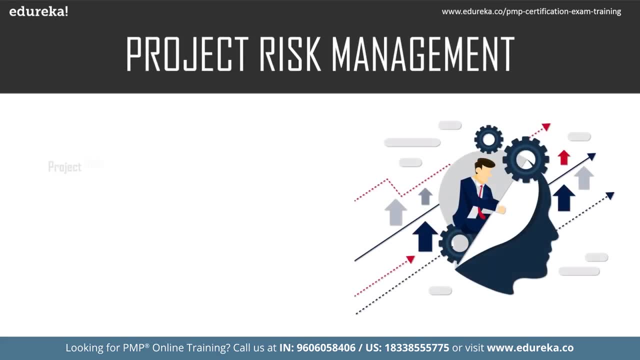 So this is the kind of responses you will get into. So project risk management focuses on risk which are associated with the project which are undertaken. So project risk management, as defined in PMP, includes the processes of conducting risk management, planning, identification, analysis, response planning, response implementation and monitoring risk of a project. 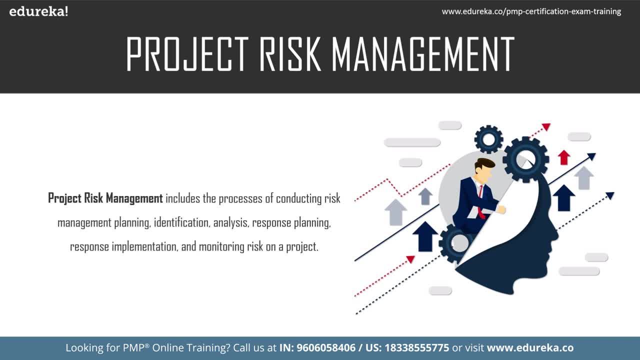 The identification of risk, analyzing the risk, managing the risk, responding to the specific kind of risk is not a one-time job. This needs to happen throughout the project life cycle. When we assess to take up a project, we identify risks. When we initiate a project, 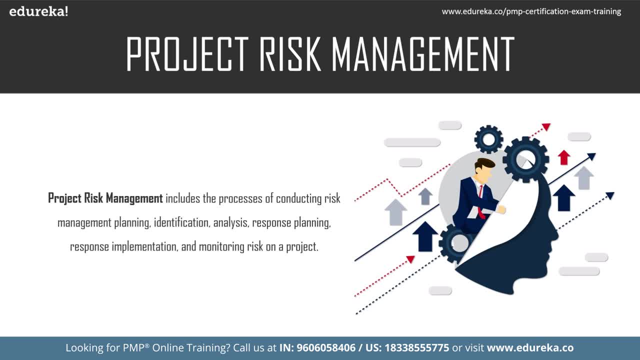 when we start the project, we identify risks. When we progress as part of the project life cycle, we identify risks, So new risks are identified and identified risks are kept analyzed at the various different parts of the project life cycle Because the impact and probability of the risk is. 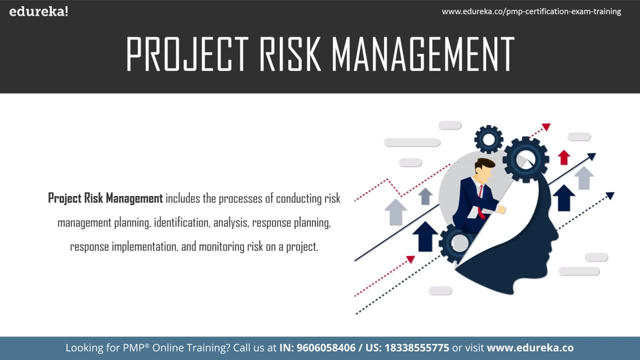 the risk, If not probability, at least impact of the risk- would vary as the project progresses, based on in what part of project life cycle we are assessing it At that given point in time. there would be variation of the risk. For example, when I begin a project. 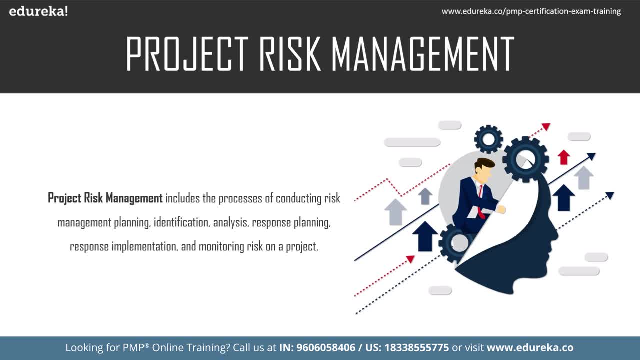 a risk like a deliverables deliverables. uncertainty is high when I start the project, But as I progress I'm ending towards the same risk. the impact will be less because the deliverables have happened in various different phases and already those are checked and tested. There is no associated risk with them in terms of a validation perspective. 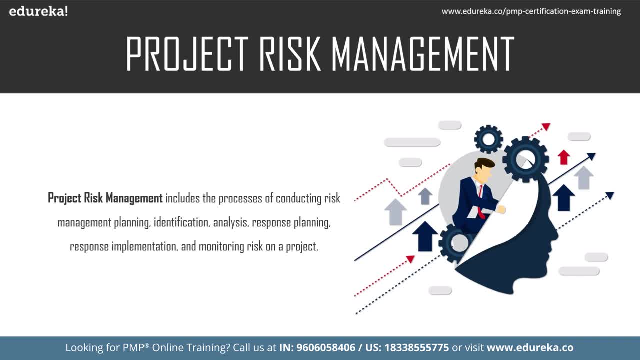 accomplishing that result perspective because majority of the deliverables have already happened. Only few deliverables will be pending as you progress towards the end of the project. So risk will be less at the end of the project. Middle of the project may be moderate. may be high. 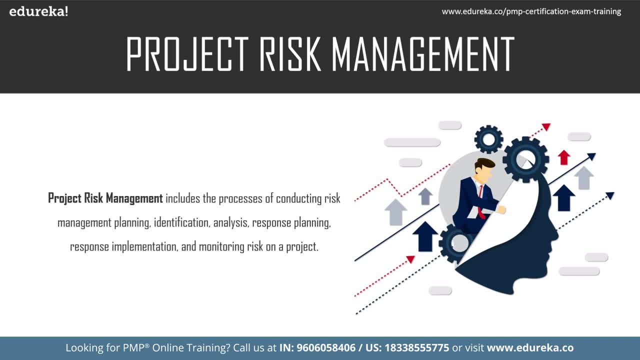 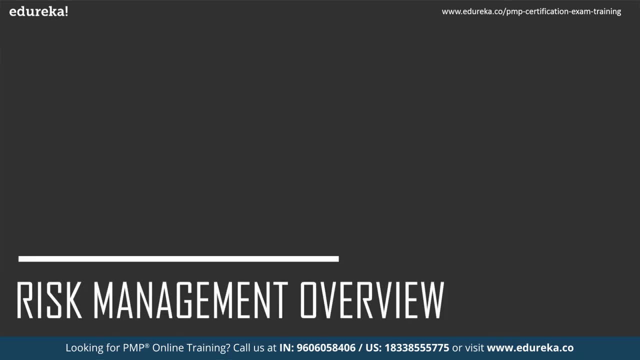 definitely not low. So likewise, for any specific risk we identify at a given point of a project life cycle, associated risk which we identified and assessed, the impact of that risk would vary. positively means increases, impact will increase or impact would decrease. So risk management overview: here we are going to look at trends and emerging practices. 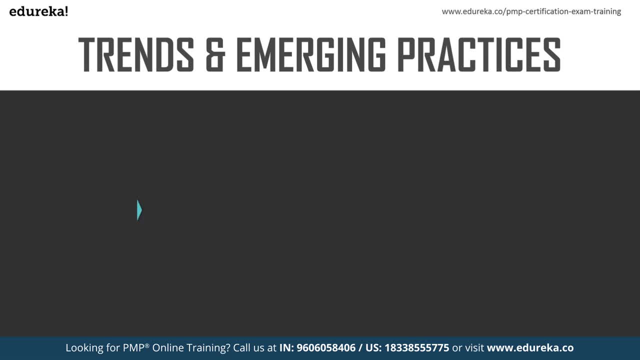 related to the risk. So risk can be looked at less like non-event risk: project resilience, integrated risk management. Now, when I say risk of something which fails, yes, that is an event, an event has occurred, So that risk we associate as an event which is associated with risk. 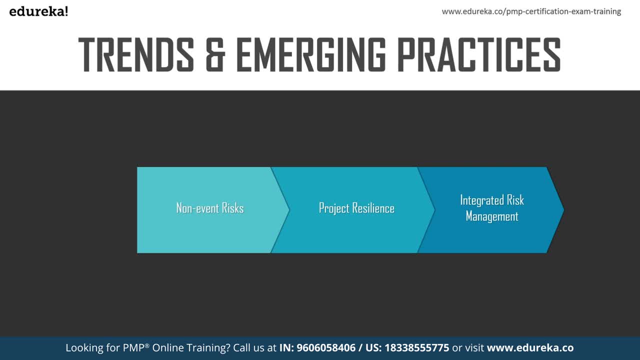 A power failure risk event, A deliverable did not happen event risk. So then, what is this non-event risk? Now, if you say I wanted to accomplish these results and these are all the benefits which has to be realized out of it, and that realization doesn't happen, that is not an 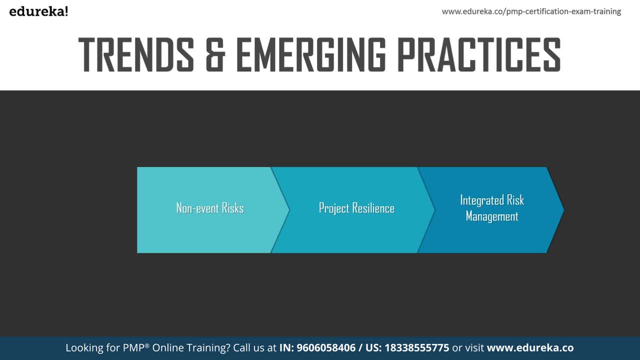 event. So because that benefit is not realized, the investment is not making sense. now This is not an event which occurred. So benefit realization happens as the product which comes as an output result should come as an outcome. That is not happening. It is not an event, it is a non-event. 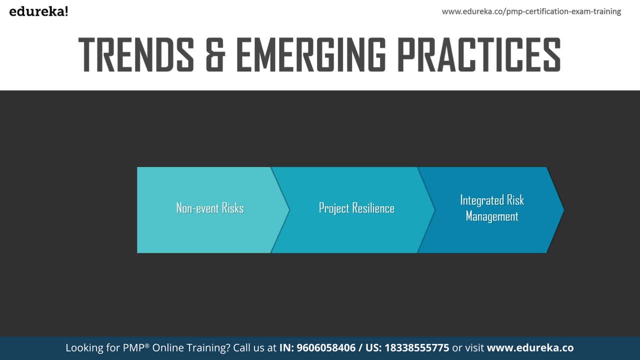 risk. People who have the specific skills and capabilities were unable to deliver properly. It is not an event. The performance of the individuals is not happening the way it is required. non-event risk. So likewise, by generic statement of risk or the definition of risk, we say: 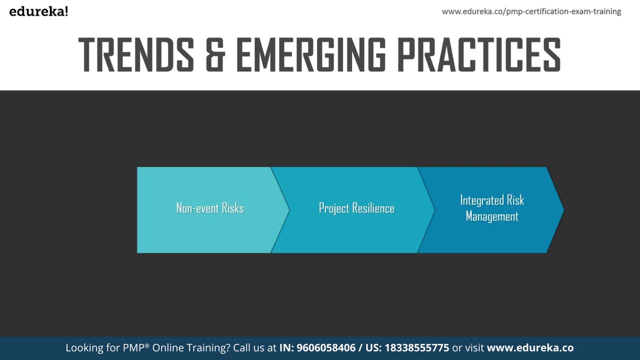 an uncertain event, for a risk, But there are risks which exist, which are non-event risks as well, which needs to be identified. Then projects resilience: Whenever a project fails, whenever there is a degradation of performance, how will a project recover? What is that ability Project as a whole could able to? 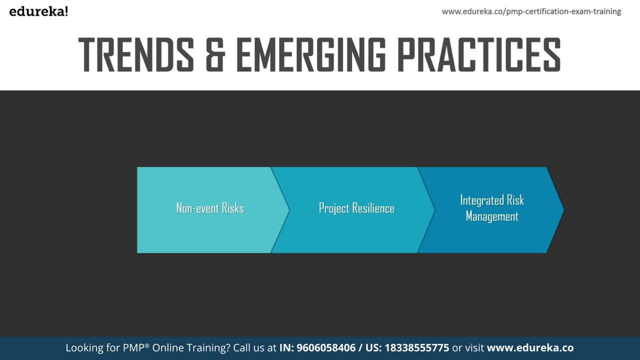 recover from it and move on smoothly further to accomplish the ultimate results. So these needs to be planned very well. Integrated risk management: So, as we know, in BMP framework we have integration management. So integration management provides an integrated view of the entire project where risk management will also go on. 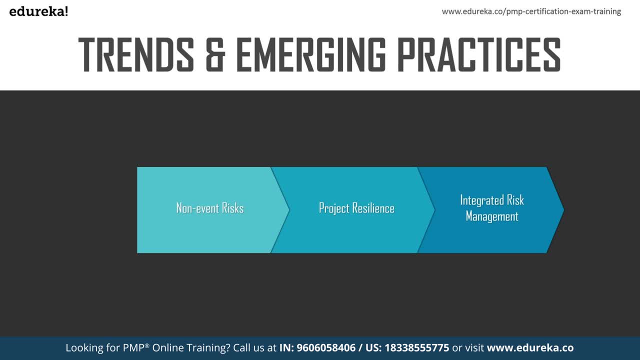 Get into that, Get integrated into ultimate project management plan. So risk management plan across the project life cycle needs to be looked at and it should have a bigger picture. It is not one or two risks, only positive or negative risk. It's about all the risks. 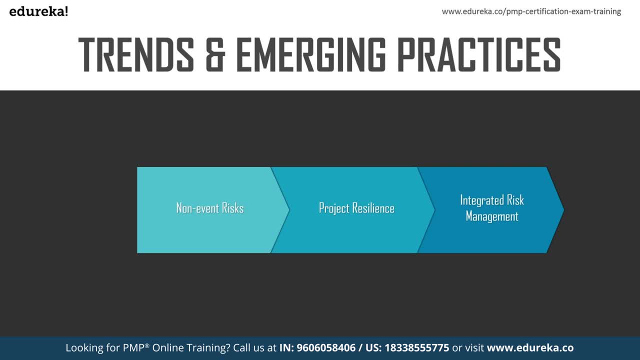 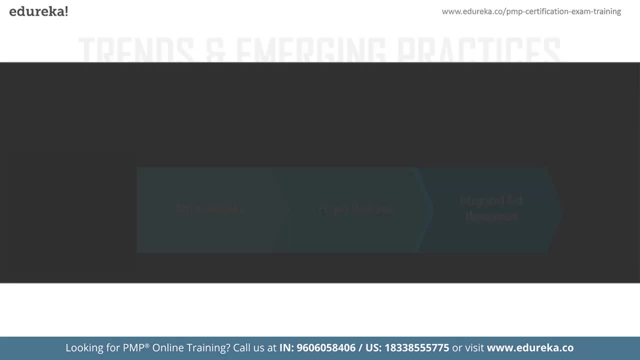 which are identified, assessed throughout and managed together. There should be a risk register to capture all of this. That is the reason there is a dedicated risk management knowledge area defined in BMP framework. So tailoring concentrations would be size of the project. 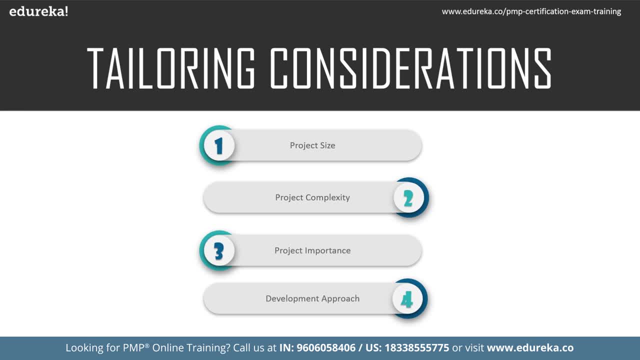 complexity of the project, importance of the project and approaches for various different things which are adapted and adopted for the project. So as the size and complexity of the project varies, obviously the impact of the projects because of certain failures will be varying. When I say importance of the project, the deliverables of the project, how important, 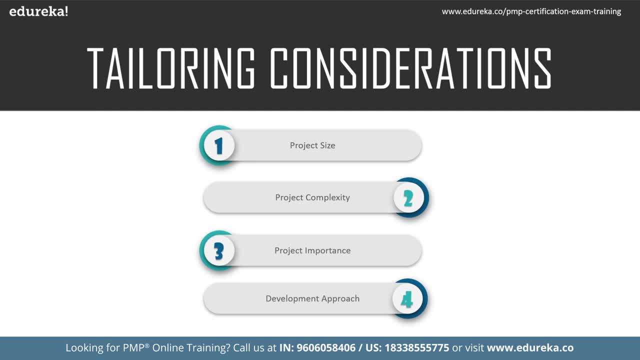 is for my business. If I am doing a project to enhance the capability of the people in general, then that is important to the business perspective, but it does not have a time target. It is a continual access for organization. But I am getting into a specific new project and I need 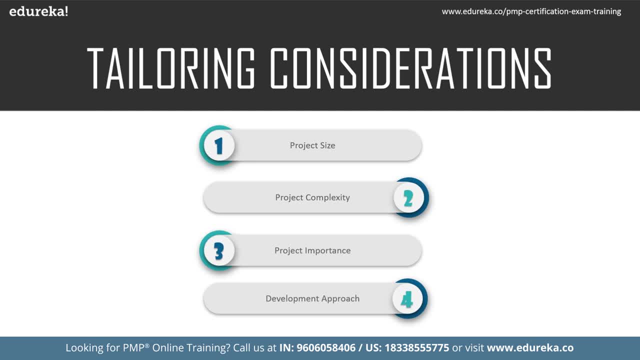 people's competency should be improved. Now I have a specific point in time before which I should have that capability, Otherwise I will lose on that opportunity. So likewise my tailoring consideration in the projects in terms of what is that I am going to deliver, what is that benefits? 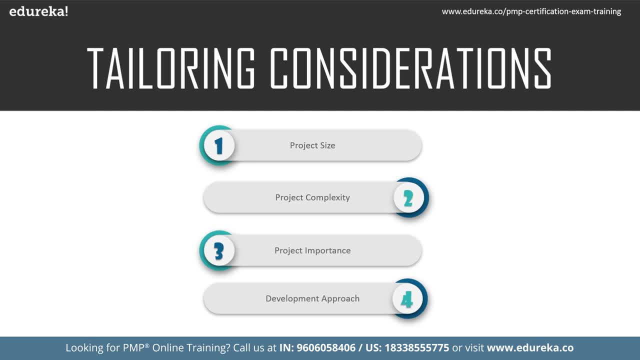 the people who are investing on this project. what is the return they would get? Unless that is visible, we cannot say how important the project is. Approaches defined would be based on what kind of technology is used, what kind of deliverables required, what kind of environment we are into, what are the outputs which should come out of a 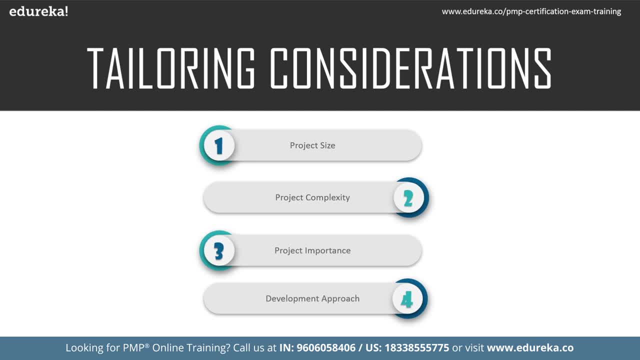 project? what would be the outcome of that project? As you define all of this, when the direction is set clearly, accordingly, one can take an approach So people can adopt a predictive lifecycle project management, adaptive lifecycle project management, which is basically a waterfall. 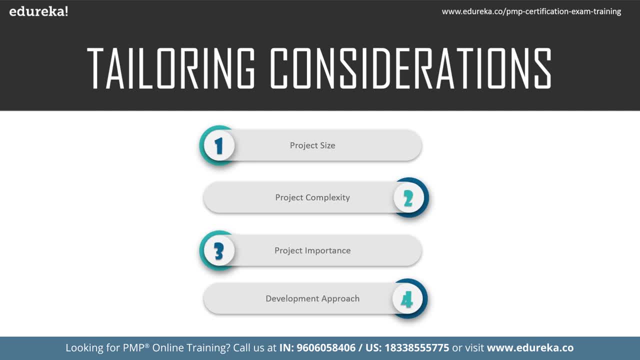 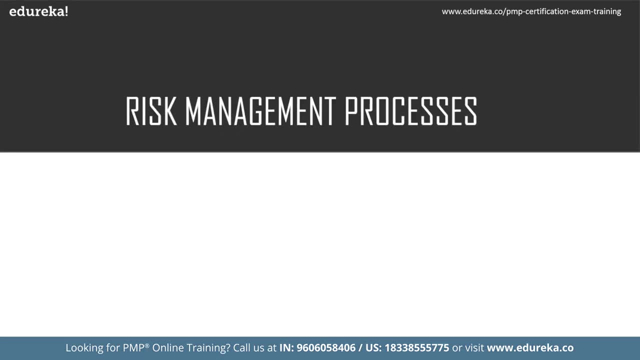 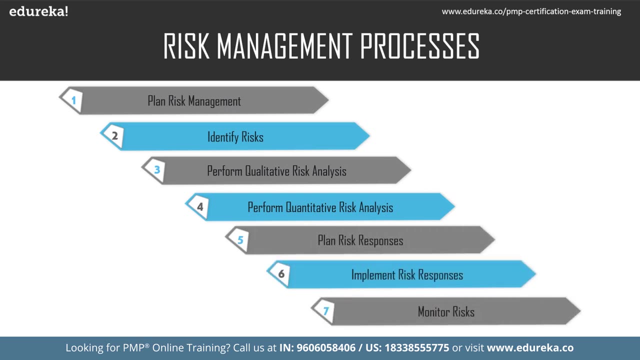 versus agile approaches, Two different approaches which we can broadly mention about. So risk management processes. So risk management processes includes planned risk management, identifier risks, perform qualitative risk analyses, perform quantitative risk analyses, planned risk responses. So all the processes 1 to 5 are part of planning process group. 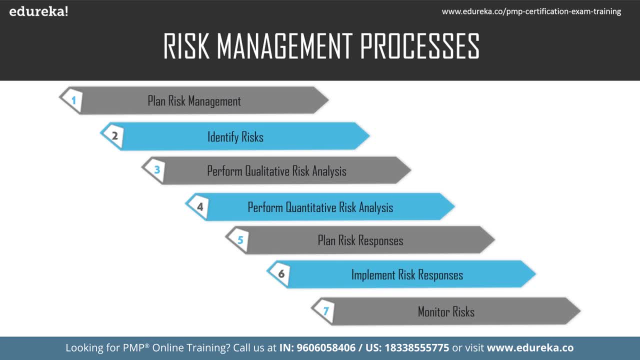 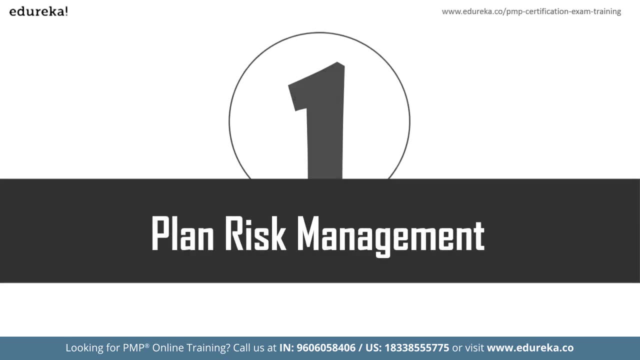 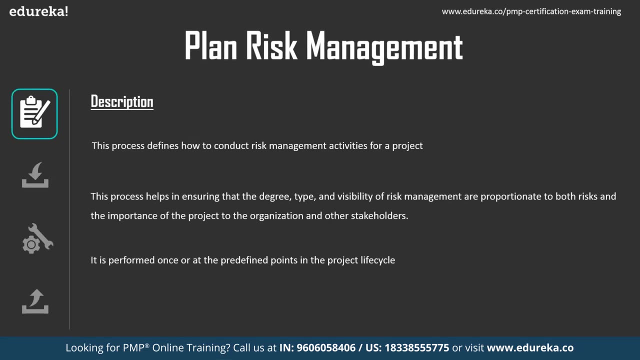 Implement risk responses will be part of executing process group and monitor risk will be part of monitoring and control process group. So planned risk management, which is the first process in this knowledge area, focuses on defining how to conduct risk management activities for a project. 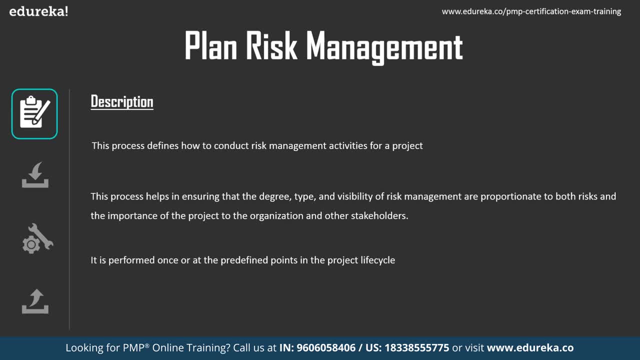 This process helps in ensuring that the degree, type and visibility of risk management are proportionate, both risk and the importance of the project to the organization and other stakeholders. So it is performed once or at the predefined points in the project lifecycle. But, however, even though it is defined in the planning process group, here in the framework, 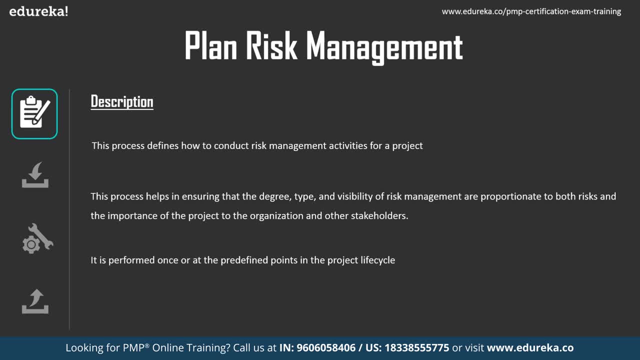 planning for the risks should be an integrated one which should be applicable to the project. So planning for the risks should be an integrated one which should be applicable to any given scenario of the project, But, however, if there is any modification for this, 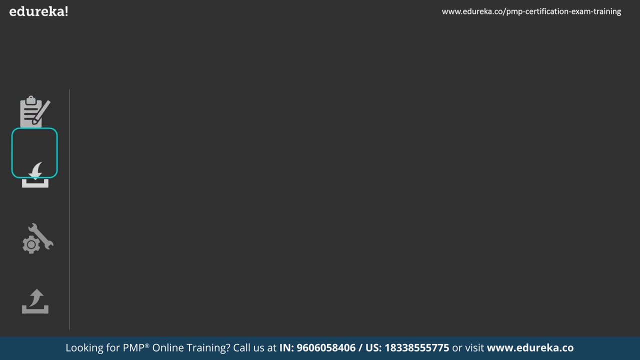 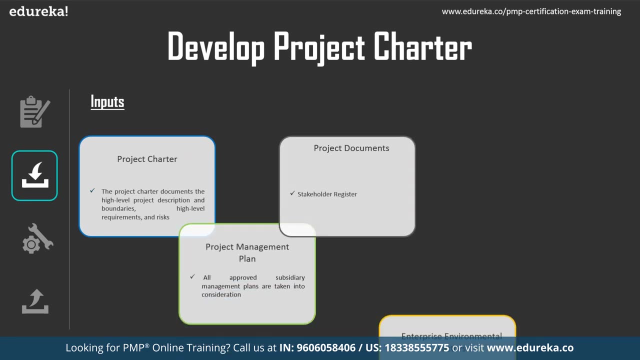 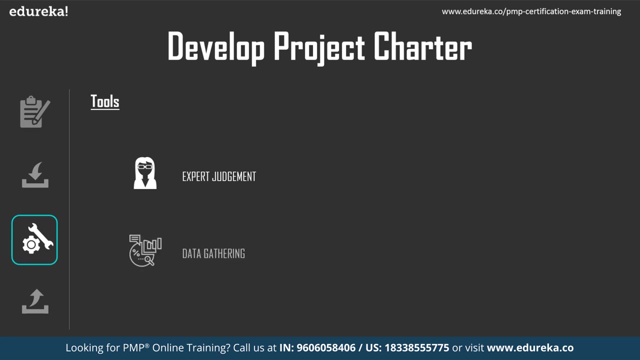 as we progress in the project required. that can be done. Inputs to plan risk management process would be project charter, project management plan, project documents, enterprise, environmental factors and organizational process. assets Tools would be expert judgment, data gathering meetings, whereas outputs would be risk management plan. 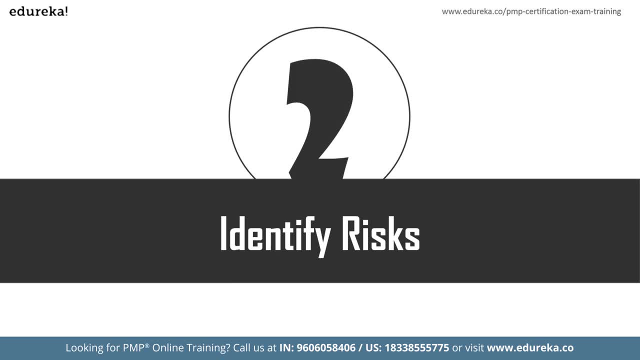 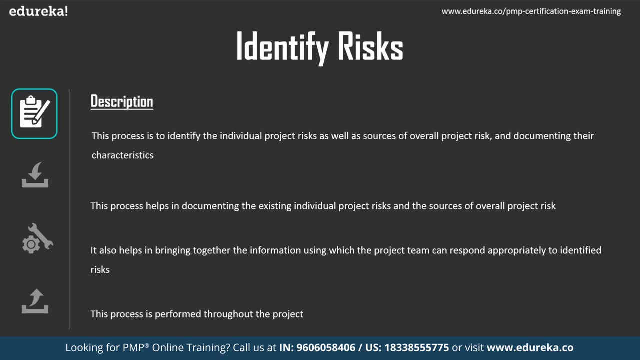 So identifier risk. Identifier risk is a process which identifies the individual project risk as well as the sources of overall project risks. So when I say sources, we're speaking about the causes of that risk and documenting those risks and all the associated details describing why. should I? 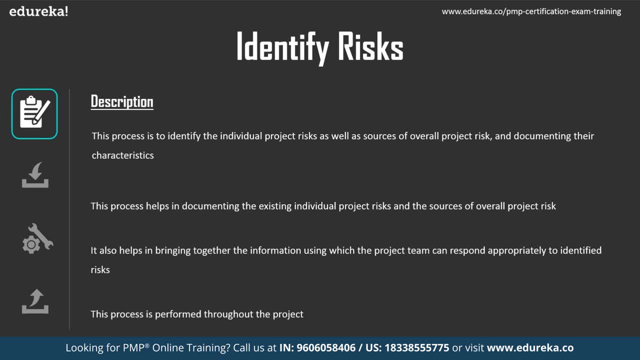 consider this as a risk. Why am I saying it is a risk That needs to be described. So this process helps in documenting and existing individual project risk and the sources of overall project risk. It also helps in bringing together the information using which the project team can respond. 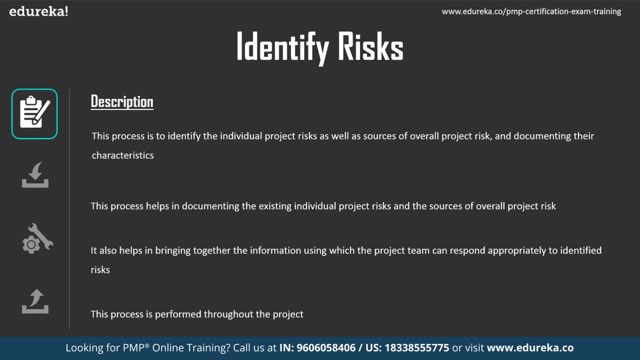 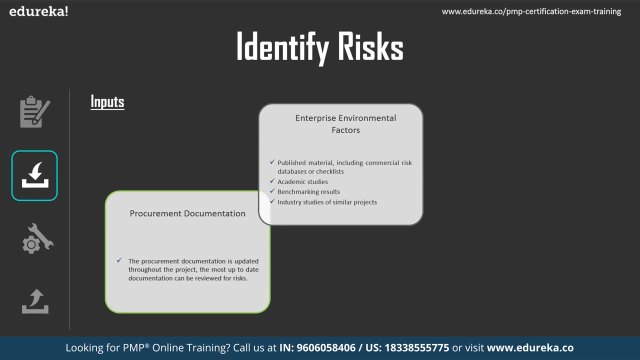 appropriately to identified risk. This process is performed throughout the project, So one has to keep identifying the risk throughout the project lifecycle. So input of identifier risk process would be project management plan, project documents, agreements, procurement documentation, EEF and OPA, Whereas tools used as part of identifier risk process would be expert judgment. 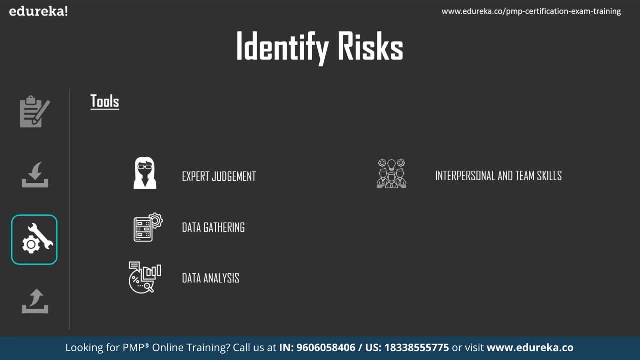 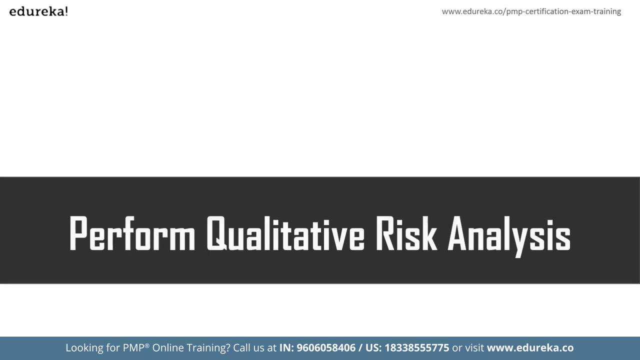 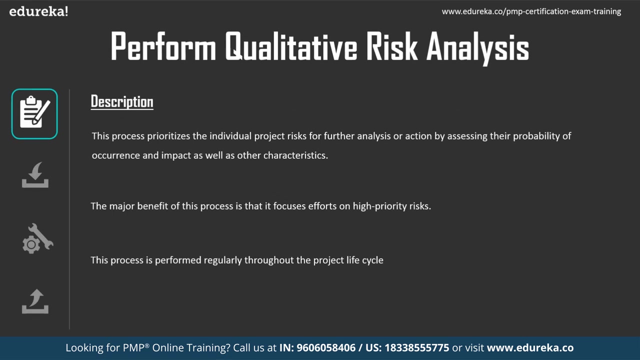 data gathering, data analysis, interpersonal and team skills, prompt lists and meetings. The outputs of identify risk process would be risk register, risk report and project document updates. The next process for us is perform qualitative risk analysis. So perform qualitative risk analysis is the process of assessing and analyzing the identified risk qualitatively. So this helps in. 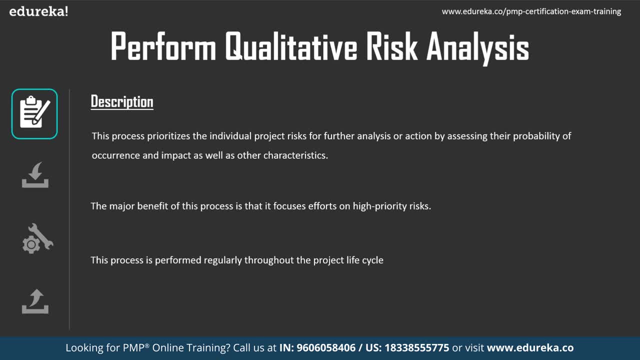 flavours the risk of the projects or acts in the activity. So, for example, if individuals are looking for delivery of 1964 products to India, If an individual is looking for delivery of 24th grade products, It may be possible to assess the risk of the products. 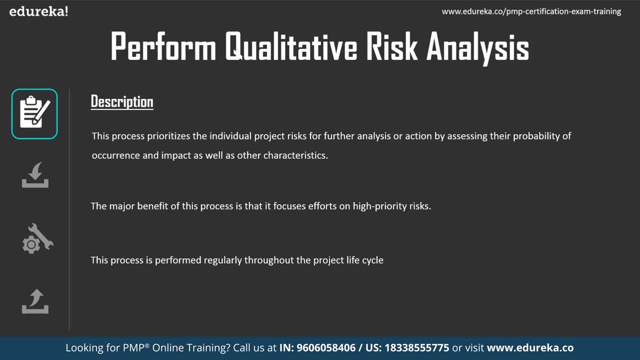 planning, processing, maintenance, inventory and physician its impact on the patient. Under this process, individual projects trace the risk and the risk of the individual projects. The process also prioritizes individual project's risk and also looks at major benefits of this process, which is the focus effort of high priority risks. These activities are done regularly. 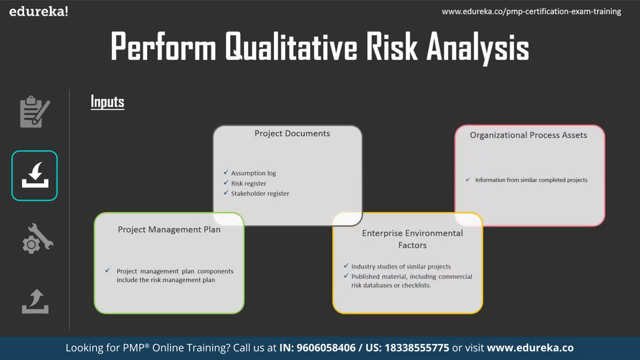 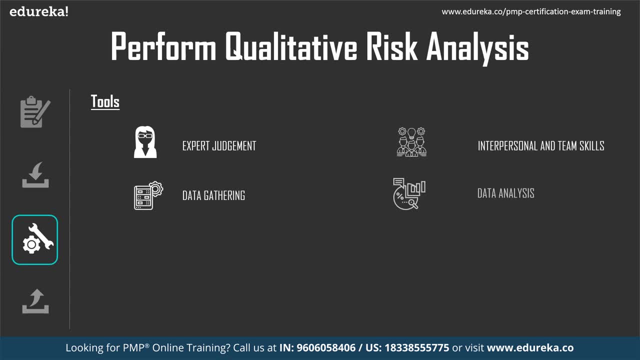 throughout the project lifecycle and inputs to the project management plan, project documents, EEF's and OPA tools. tools used: our expert judgment, interpersonal and team skills, data gathering, data analysis, risk categorization, data representation and meetings so the output of this particular process, perform qualitative. 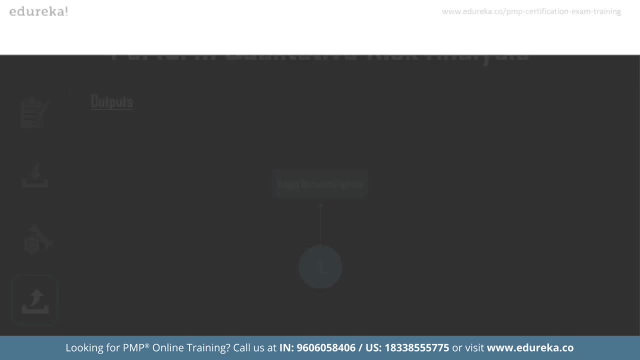 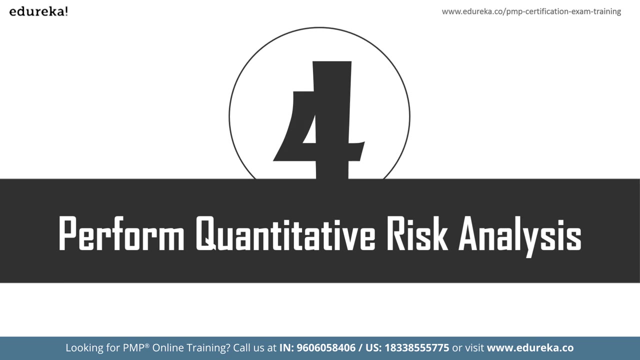 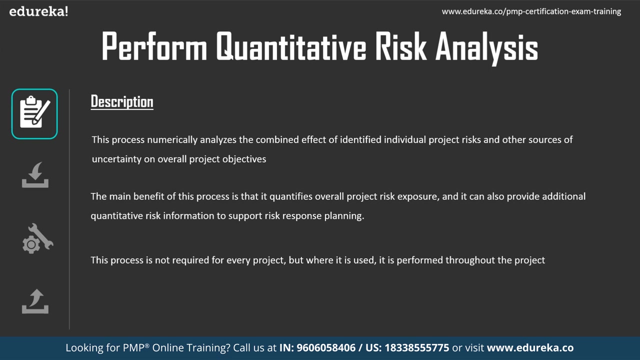 risk analysis would be project documents updates, so perform quantitative risk analysis. so further as after doing qualitative risk analysis, if a risk also needs to be analyzed quantitatively, so one can conduct quantitative risk analysis. so this process numerically analyzes the combined effect of identified individual project risk and other sources of uncertainty on overall 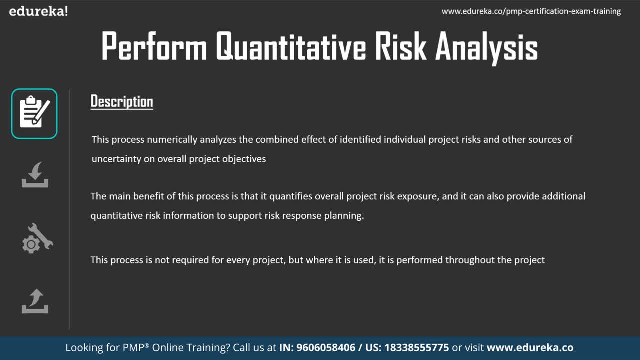 project objectives. the main benefit of this process is that it quantifies overall project risk exposure and it can also provide additional quantitative risk information to support risk response planning. this process is not required for every project, but it is used. it is performed throughout the project, so where should we use this? 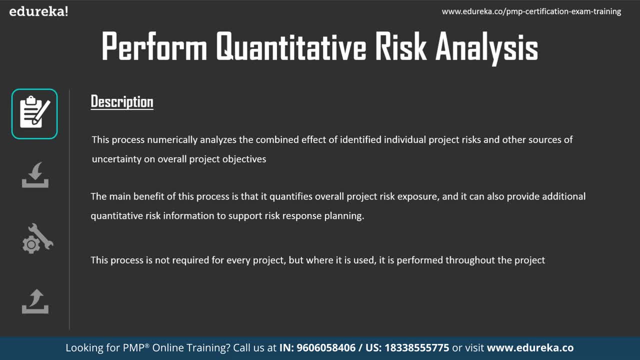 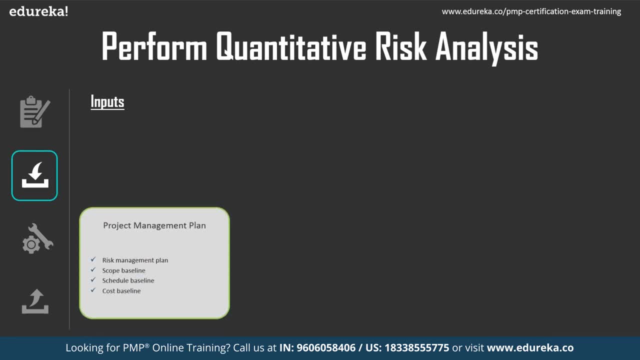 quantitative risk analysis wherever the project size is big, where the project is complex. so inputs to this particular process would be project management plan, project documents like assumptions log, basis of estimates, cost estimates, cost forecast, duration estimates, milestone lists, resource requirement, risk registers and schedule forecast. so enterprise, environmental factors as well as OPA. so tools used as part of this particular 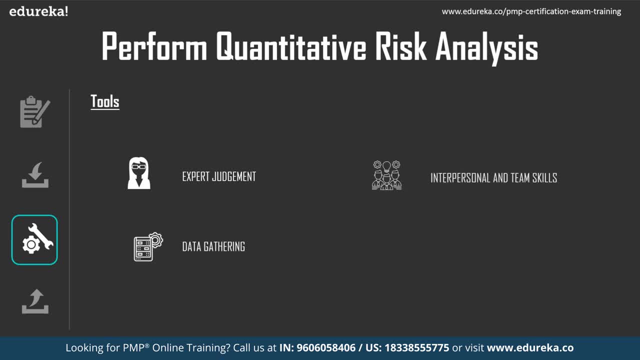 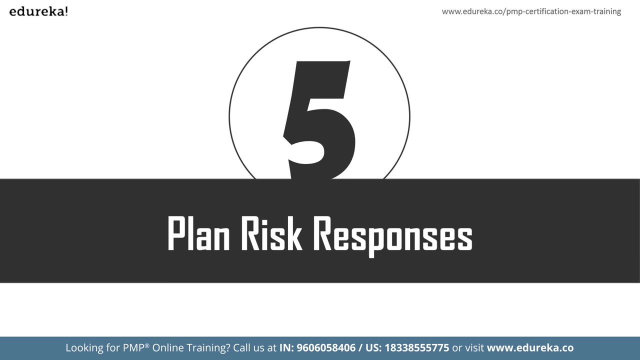 process would be: expert judgment, data gathering, interpersonal and team skills, representation of uncertainty. then data analysis, the outputs, project documents, updates, so planned risk responses, so as we identify the risk and then analyze them qualitatively and quantitatively, so we know positive risk or negative risk, what kind of impact each of those risk would. 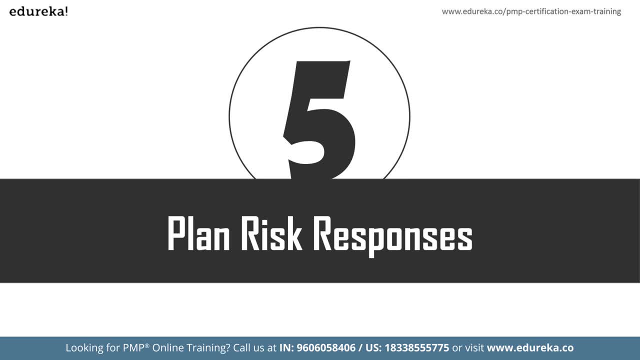 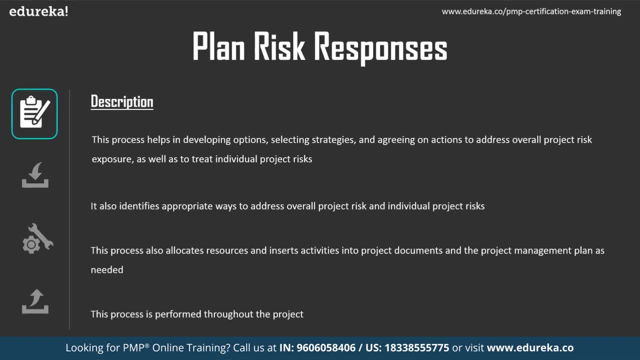 have. so how are we going to get benefit of positive risk? how are we going to reduce the impact of negative risk? so this requires planning risk responses. so this process helps in developing options, selecting strategies and agreeing on actions to address overall project risk exposure, as well as to treat individual. 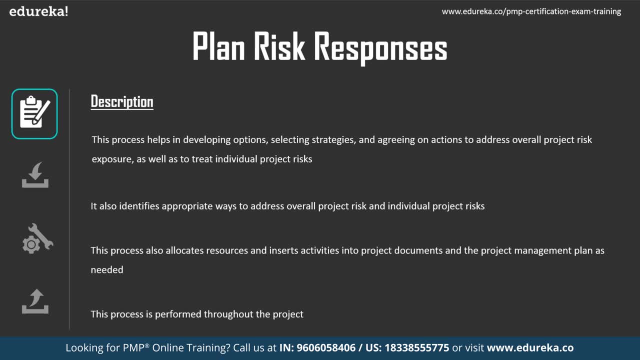 project risk. this also identifies appropriate ways to address overall project risk and individual project risk. this process also allocates resources and inserts activities into project documents and the project management plans as needed. so this is performed throughout the project lifecycle. so now inputs to planned risk responses would be project management plan, which involves resource. 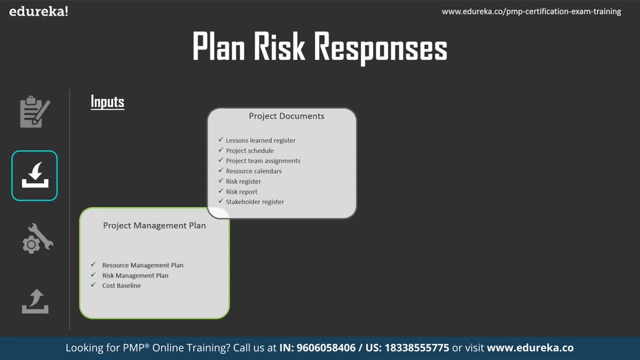 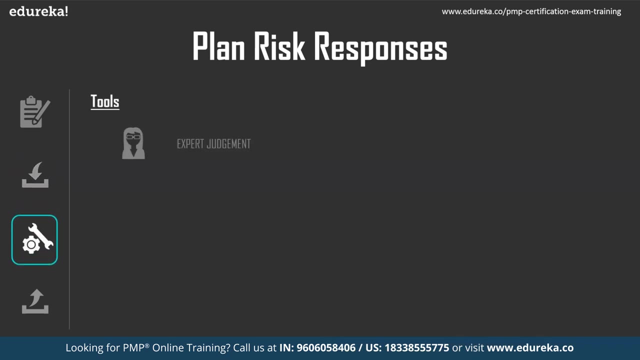 management plan, risk management plan and cost baseline. then project documents, which is lessons learned register, project schedule, project team assignments, resource calendars, risk register, risk report, stakeholder register, EF and OPA. tools for tools. tools involves expert judgment, data gathering, interpersonal and team skills. strategies for threats, strategies for opportunities. then contingency response. 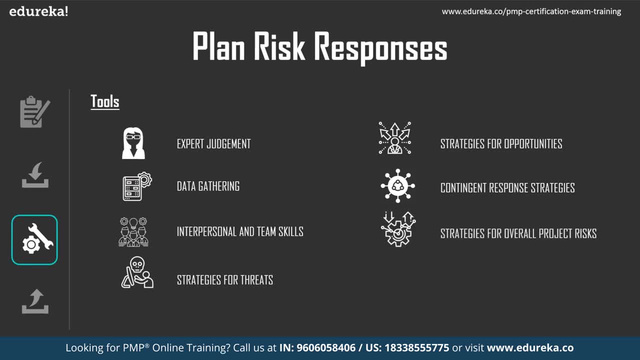 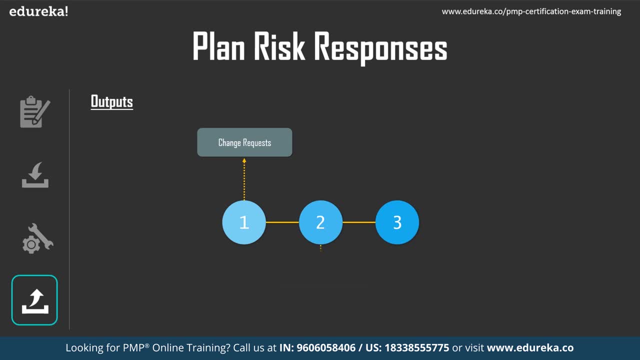 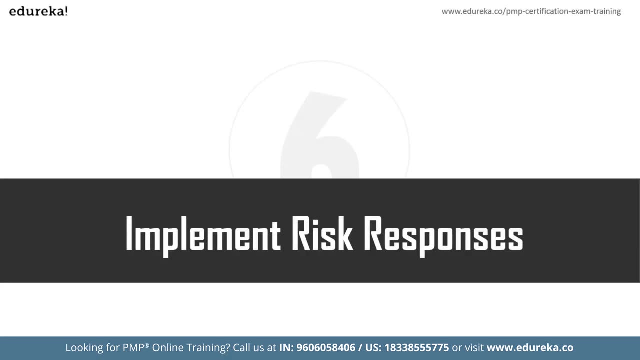 strategies, strategies for overall project risk data analysis and decision making. the outputs of this process would be change request, PMP updates, that is, project management plan updates and project documents updates, so implement risk responses. so as we plan for risk responses, it is very essential for us to look at 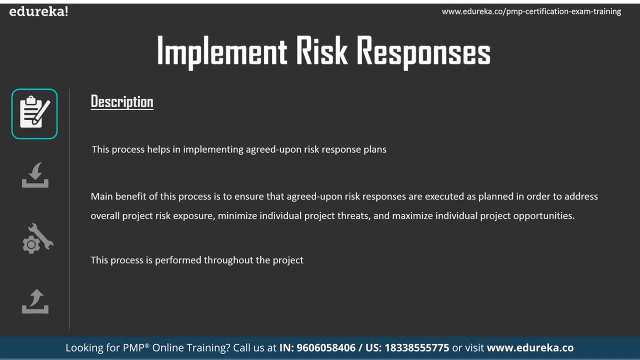 implementation of that responses. so this process considers all those risk responses, plan what is defined already and accordingly it will implement. so this process of implementing agreed upon risk response plans provides the key benefit. so what is the key benefit of this process? that is, to ensure that agreed upon risk responses are executed as planned in order to address overall. 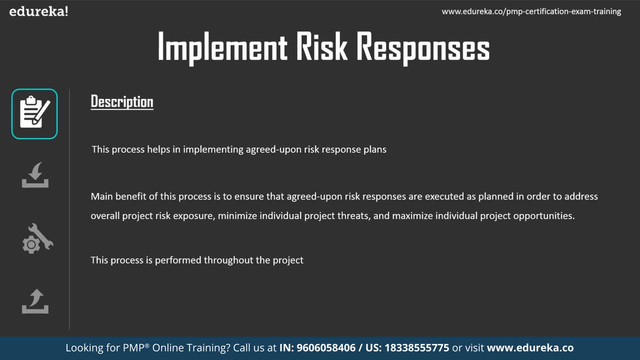 project risk exposure exposure minimizing the individual project threats and maximizing overall project opportunities. So process helps in implementing agreed upon risk response, as I mentioned earlier. So now, once we are ready, we are making ourselves ready to respond to the risk scenario. Some of the risks you cannot even able to reduce by doing the risk response plan implemented. 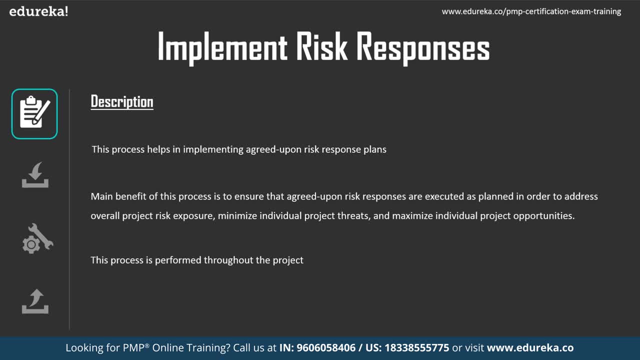 If power going off in between, while you are playing, presentation or conducting a training, so that will impact the training. So how will you ensure the power is available always? So you will go for UPS. That is a response plan, what you made. So UPS cannot give the backup more than 2 hours, 3 hours. 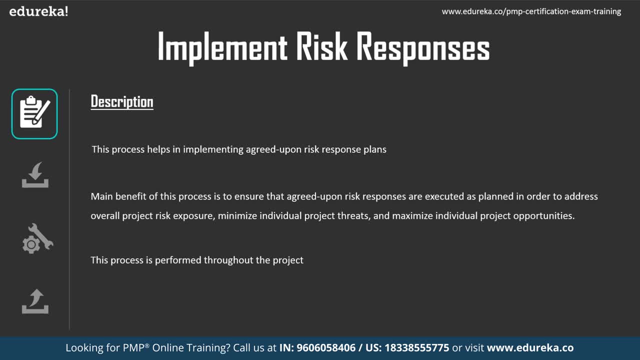 Let us assume that You will have a generator so that if power fails, UPS will take care immediately. Then you go and switch on the generator which will generate the power, and load on the UPS would come down And UPS is always in the loaded condition so that even generator fails, UPS will take care for some time. 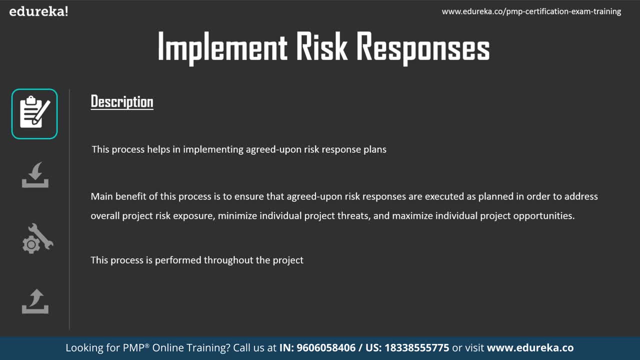 But there will be some scenarios where fuel is not available, So generator cannot run. So such risks are called residual risk, which we will accept Because we implemented this UPS as well as generator. it is quite obvious these two introduces additional risk: Risk associated with UPS itself, risk associated with generator itself. We call it as a secondary risk. 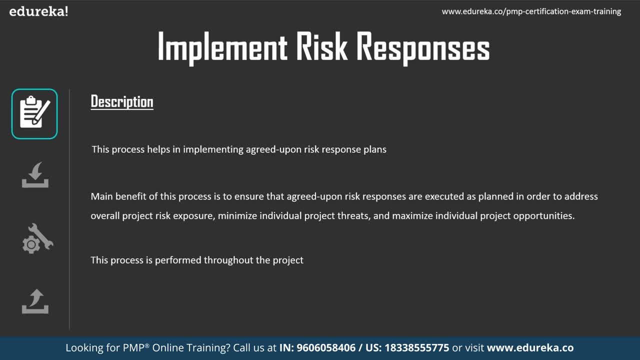 So in this case, what we did was, before the occurrence of the risk, we implemented the risk responses. But there will be some scenario where you cannot implement the risk responses. You should yourself make ready to handle those scenarios. What if the building collapses? 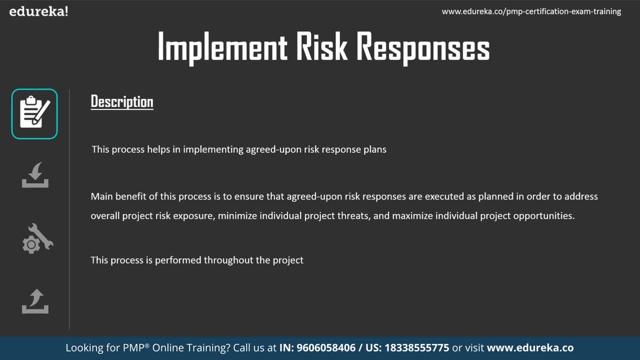 What if earthquake happens? What if flooding happens? So you will have a contingency plan defined. So contingency plan you can implement, Or else looking at the impact kind of thing, you will make yourself ready, Let it go. I have other modes of operating my business and move forward or make my project successful. 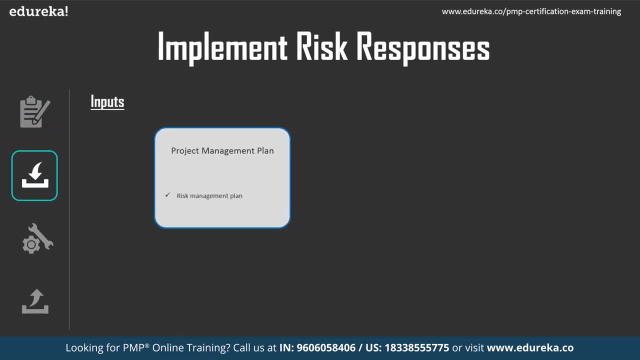 So inputs to this particular process would be project management plan, project documents and OPA. Tools used as part of this particular process is expert judgment, interpersonal and team skills project management information system. Outputs would be project document updates and change requests. 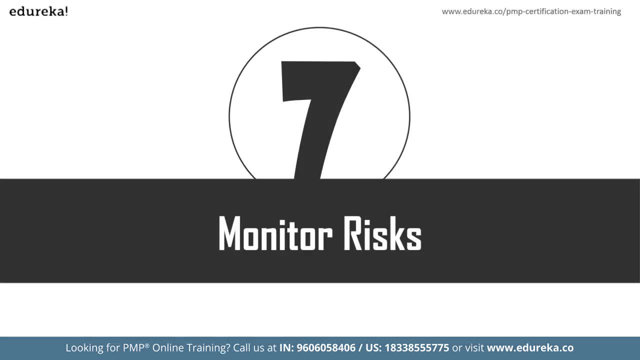 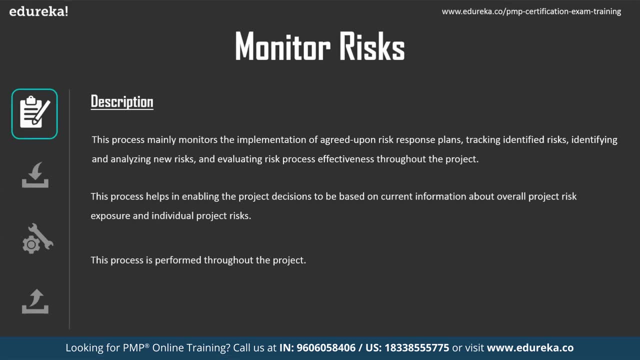 Monitor risk process- Monitor risk process, which is part of monitoring and control process group defined in PMP. This process mainly monitors the implementation of agreed upon risk response plans, Tracking identified risk, identifying and analyzing new risk and evaluating risk process effectiveness throughout this process. 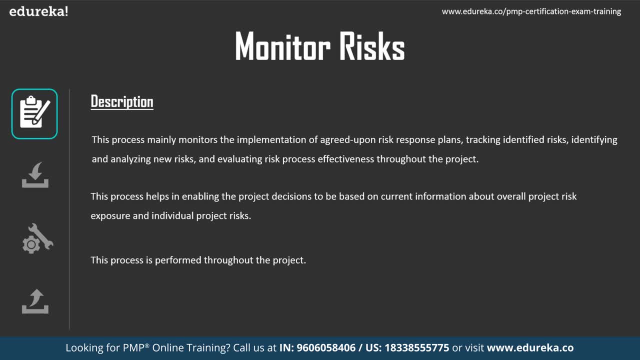 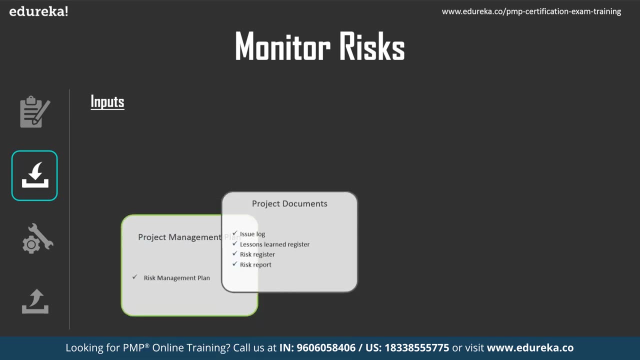 So this process helps in enabling the project decisions to be based on current information about overall project risk exposure and individual project risk. So this is performed throughout the project lifecycle. So input to this process would be project management plan, project documents, work performance data and work performance reports.